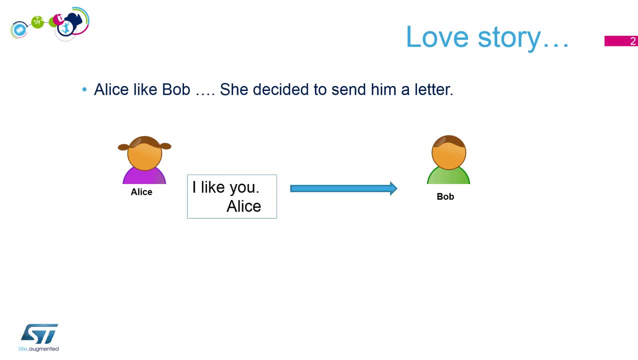 So she writes: I like you, just sign Alice and send this to Bob. Unfortunately, we've got Eve and Eve can't stand Alice, So she managed to intercept this message. She modified it- I dislike you. and now keeps the signature of Alice and sends this to Bob. 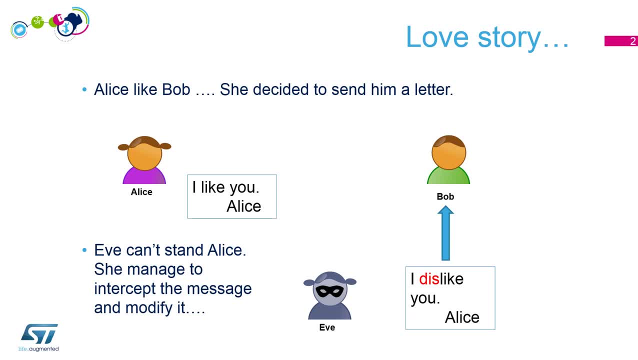 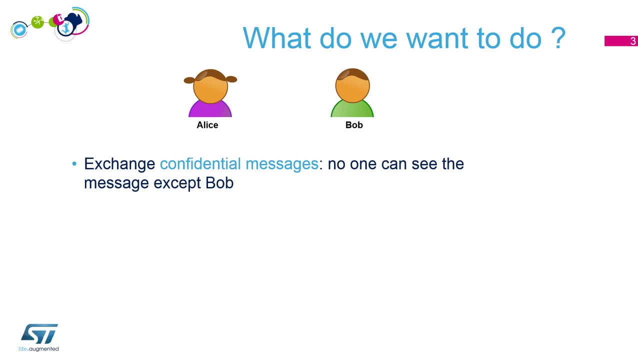 What a shame. How can we help Alice and Bob First, what do we want to do? We would like to have the confidentiality of the message. That means we want to be sure that only Bob can read these messages coming from Alice, Nobody else. 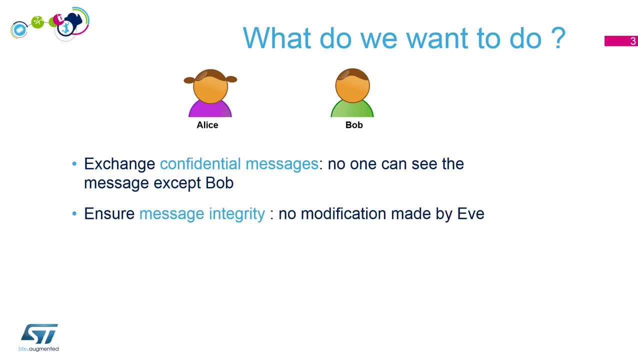 The confidentiality of this message. Then we want to keep the message integrity. We don't want Eve to be able to modify this message Or we don't want Bob to be aware about any modification. This is the message integrity. And the last point: we want authentication. That means Bob wants to be sure the message is coming from Alice and not from somebody else. 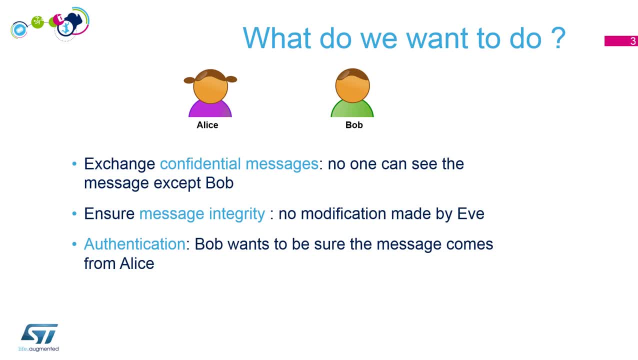 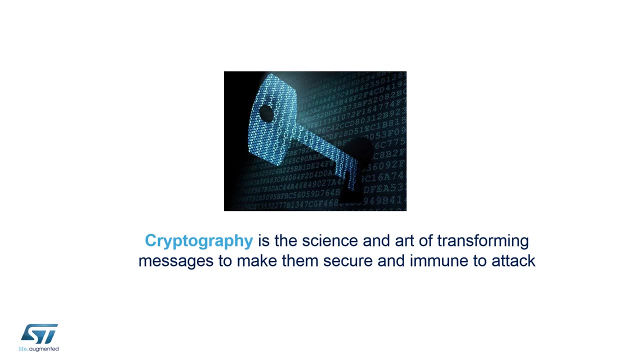 So let's see how we can address these three points: Confidentiality of the message, Message integrity, Authentication. And this thanks cryptography. Let's start with the definition of cryptography. It's a science and art of transforming messages to make them secure and immune to attack. 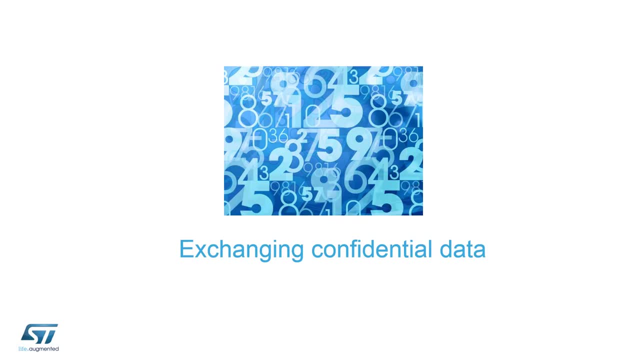 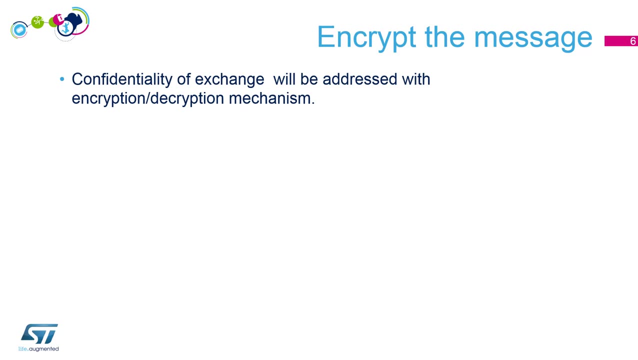 The first point we want to address. it was the confidentiality of the message. For this we will need to encrypt the message, So it was encryption. decryption mechanism will be used to address the confidentiality. There is two main categories for this: Symmetric and asymmetric one. 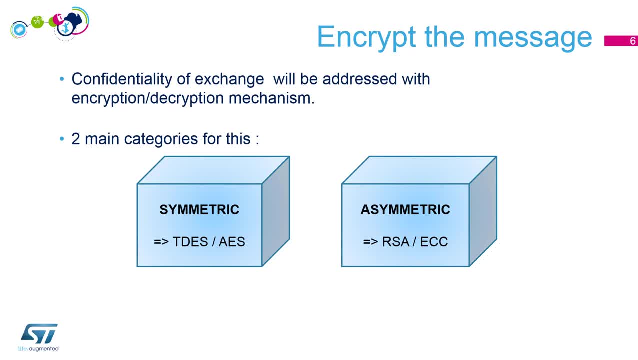 Here you've got the name of some algorithms and we will come back with details about them. About encryption and decryption, we will need keys. In this MOOC, we won't address how to protect those keys, but only how we use it. Our agenda: 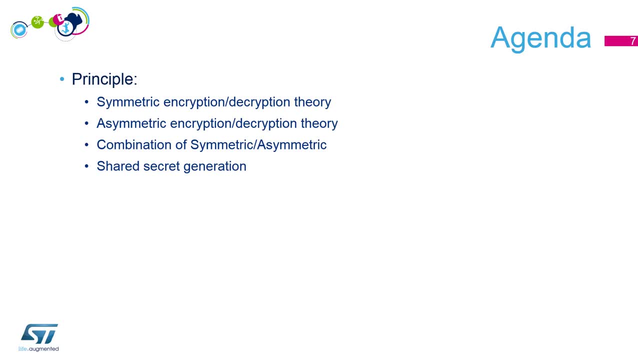 First, the principle About the symmetric, asymmetric: encryption, decryption, Then the combination of the both And how we can generate a shared secret. Then we will talk about main algorithm. For the symmetric, it will be the triple desk And how else. 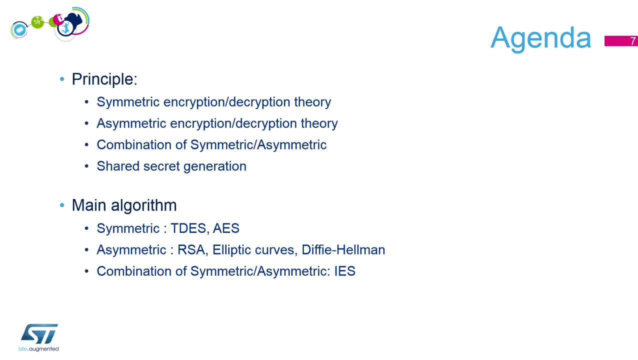 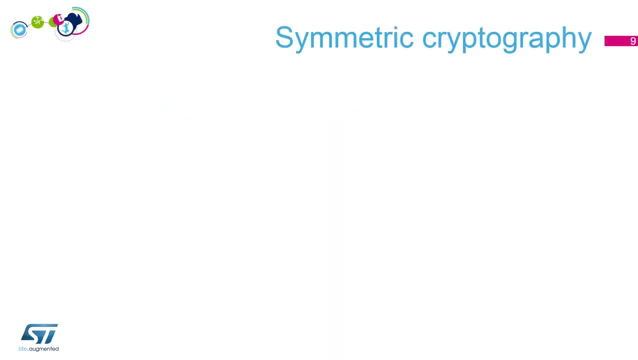 For the asymmetric, we will talk about Eressa, Adeptic curves and Diffie-Hellman, Then the combination of the, both Encryption and decryption theory. Let's start with the symmetric cryptography. In this case, Alice and Bob will need to share a single common secret. 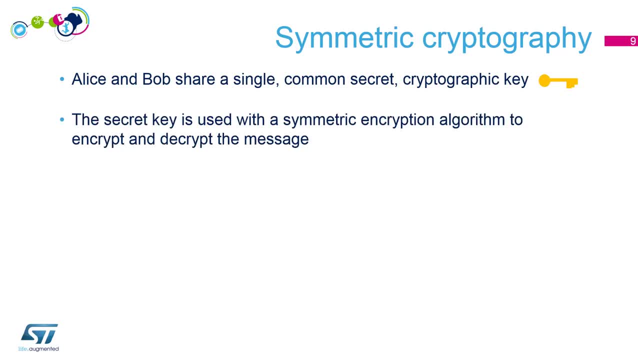 It will be a cryptographic key, The golden one. With this key, we will encrypt the message, but also decrypt the message. It's why we are talking about symmetric cryptography. It was the same key used to encrypt and decrypt. So, Alice, prepare this letter. 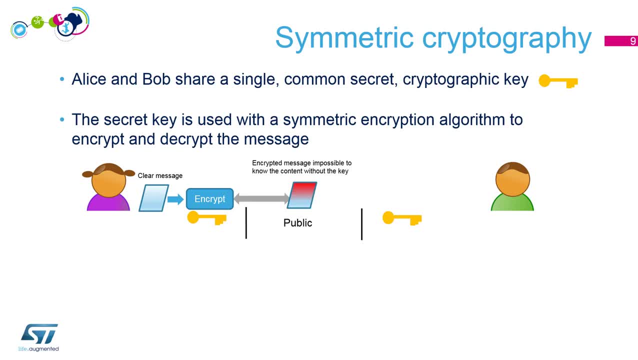 Use the key to encrypt the message And send it to Bob. At this stage, the encrypted message can be decrypted only by the one who've got the key, And Eve don't have it. So it's good Bob got this key. 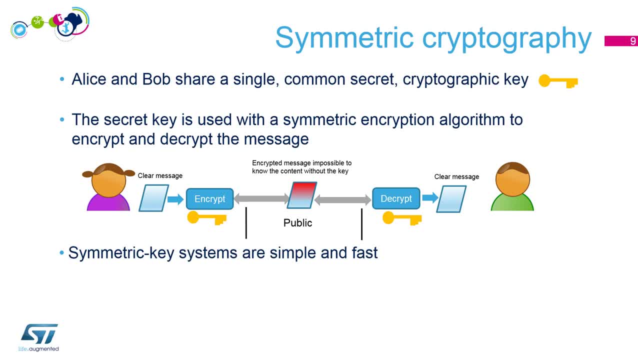 He can decrypt the message and get access to the clear content. Symmetric key systems are simple and fast. That means you can encrypt a huge volume of data with really good performance. But the main drawback is, before exchanging any data, you need to exchange the key and do it in a really secure way. 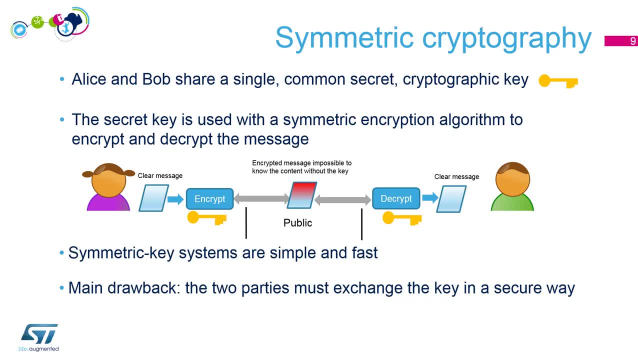 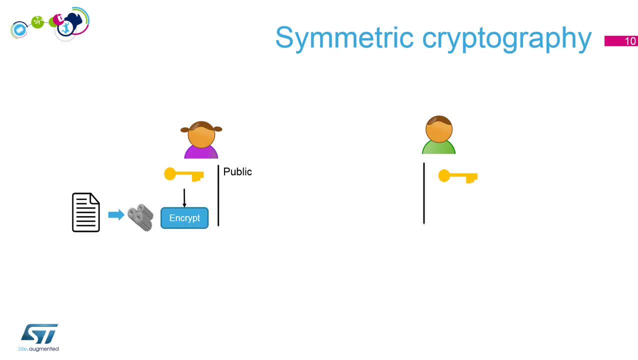 You must ensure that Eve don't manage to intercept this key. Let's fix the idea again: Alice write this letter, Use a key to encrypt the message And send this message encrypted to Bob. Bob got exactly the same key than Alice. 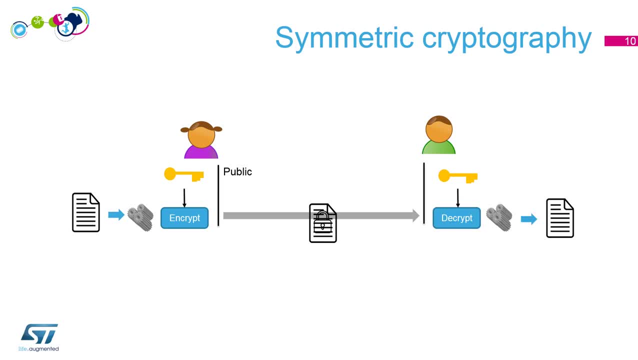 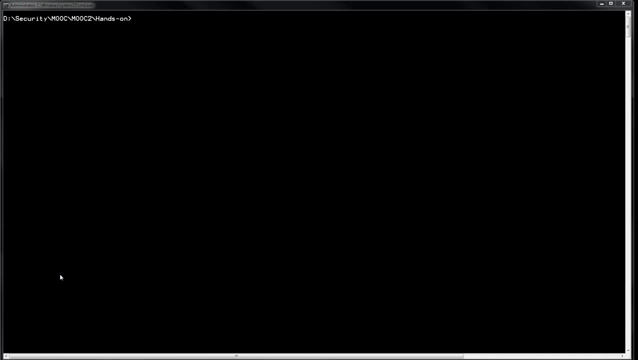 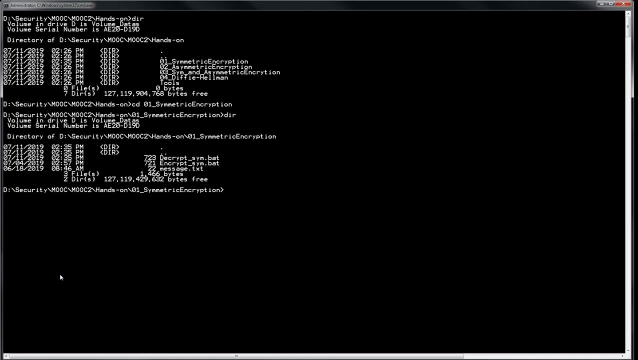 He can decrypt the message and get access to the clear content. Let's do a short hands-on to fix Heidi. So let's start the first hands-on. So I've prepared for you different folders. Let's move to the first one. So you've got a bad file to encrypt. 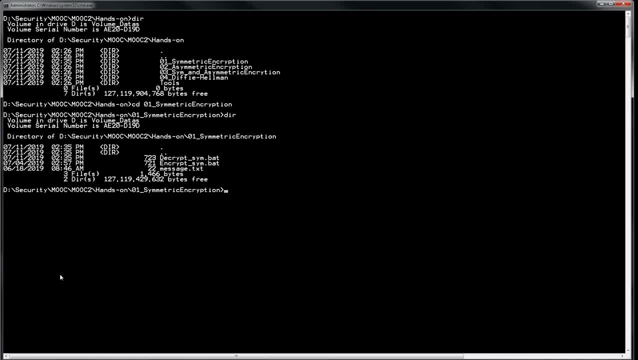 Another one to decrypt And I also provide you a message that you can modify. So if we check this message content, Dear Bob, I like you, So now let's encrypt it. So we'll call the encrypt. The first argument will be the key value. 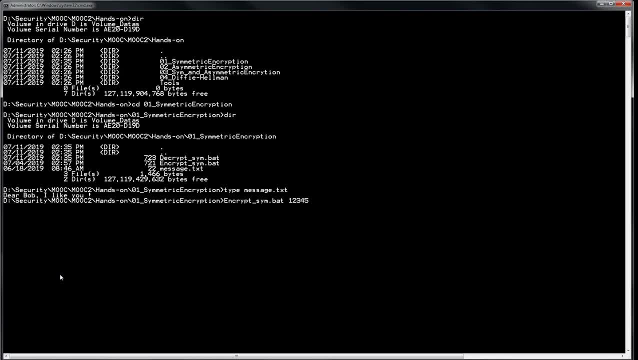 1,, 2,, 3,, 4, 5, for example. Then we'll put the message file And then the output name of the file. Let's call it encrypted, So the batch just displays you the input message. Dear Bob, I like you. 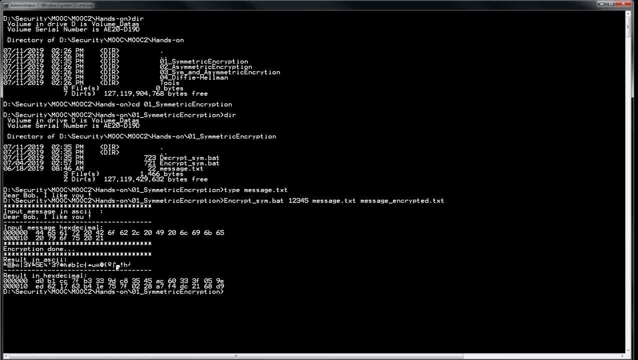 In the husky mode, In the hexadecimal. Then you can see the result in the hexadecimal of the encryption, and in the husky You can't find any information for sure. So we are in a symmetric cryptography, So we will use the same key to decrypt. 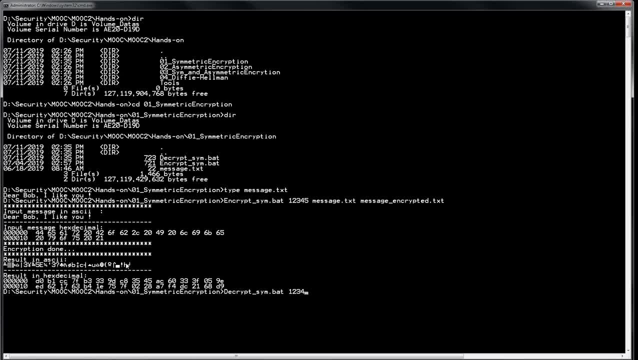 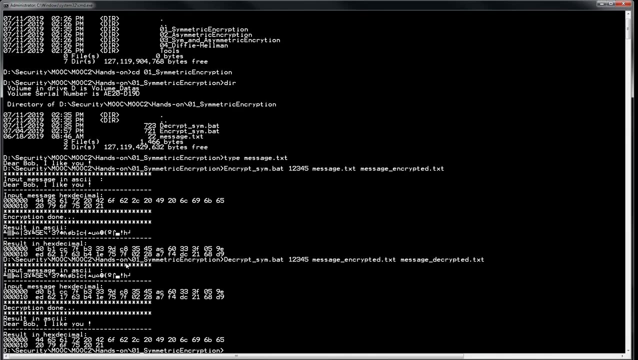 Decrypt. Let's put the same key, The input file, now with the message encrypted, And we will get the message Decrypted And the result? Dear Bob, I like you, So it was working well. OK, If I try with another value of key. 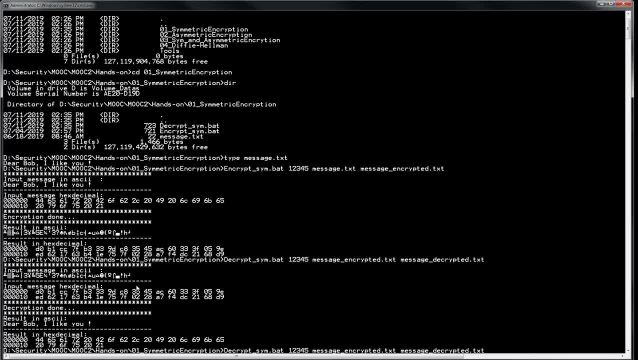 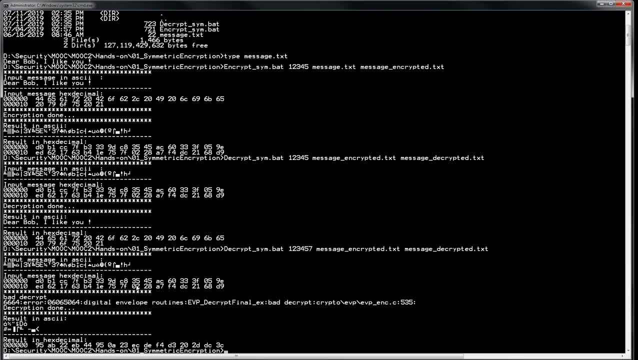 For example, I modify my key value to this. You see an error and there is some problem Here. you've got an error due to the internal tool, OpenSSL, But I would say it won't work. The values are not good, So this is really bad, but it's just to fix you, Heidi. 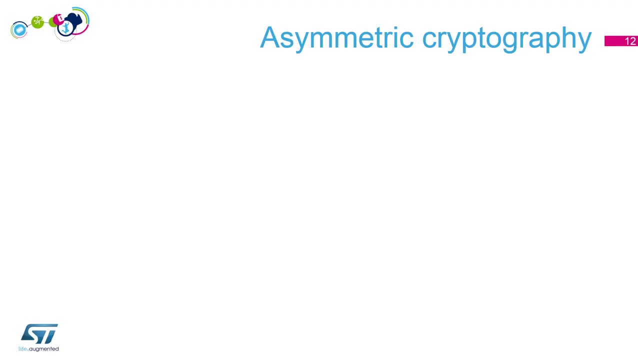 Let's continue with the asymmetric cryptography. Now encryption and decryption will be done with different keys. That's explaining the name of asymmetric. Bob and Alice have a key pair, So Alice got her key pair, Bob his key pair. We'll see that there is a public key associated with a private key. 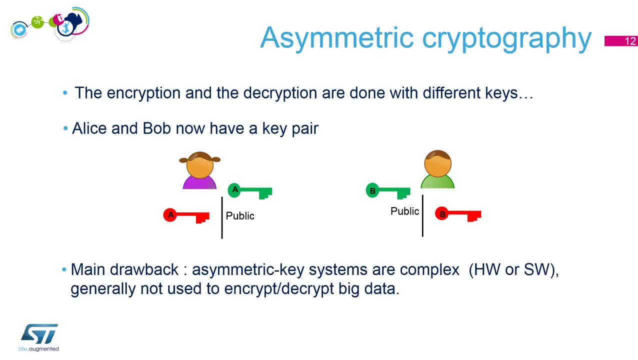 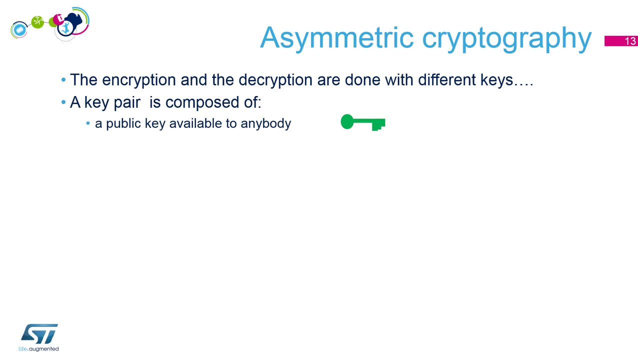 The main drawback of asymmetric key systems is the complexity. I mean it's very difficult to encrypt a huge volume of data in an efficient way, So it's usually used for tiny data. So a key pair is composed of a public key, So public means it's available to anybody. 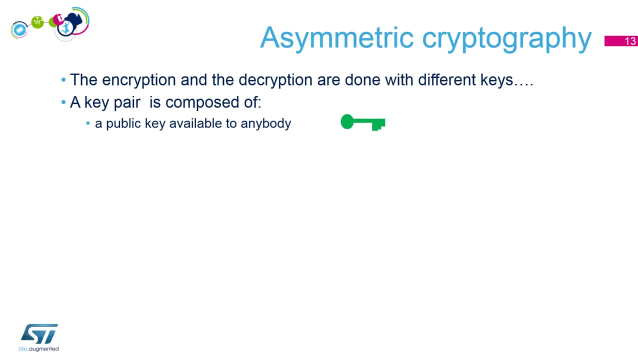 Keep this in mind. A public key is really public. A private key should be kept secret for sure, And they are linked together since mathematical properties. If you encrypt them, if you encrypt something with a public key, you can only decrypt it with the associated private key. 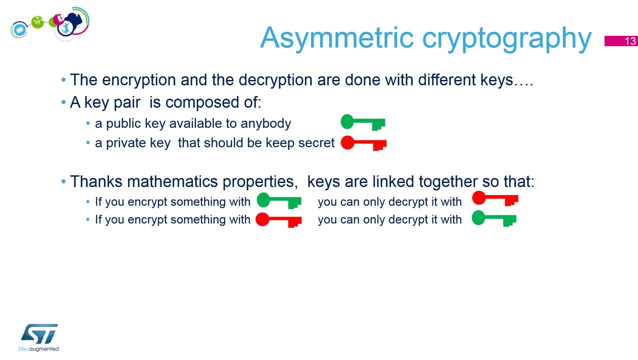 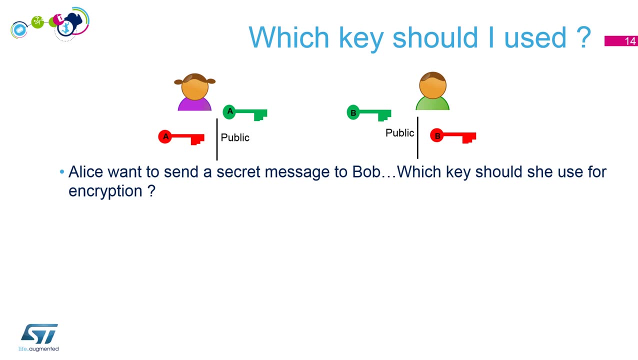 And symmetrically. if you encrypt something with a private key, you can only decrypt it with a public key. So let's see how we can use this. Alice is ready now to, I would say, encrypt the message to Bob, And the question is: which case should she use? 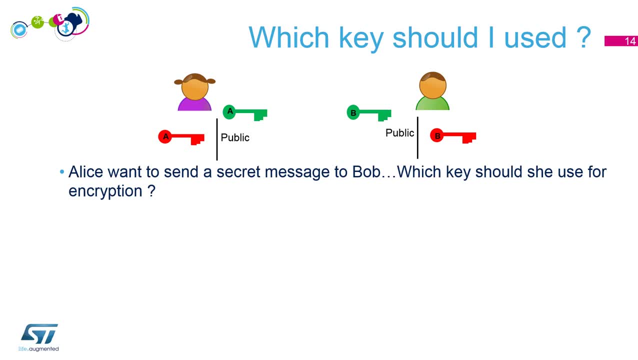 Alice got access to three keys in the schematics: A private key, a public key and the Bob public key. So let's try all the keys. If Alice encrypts with her private key, we can decrypt this message with the associated public key. 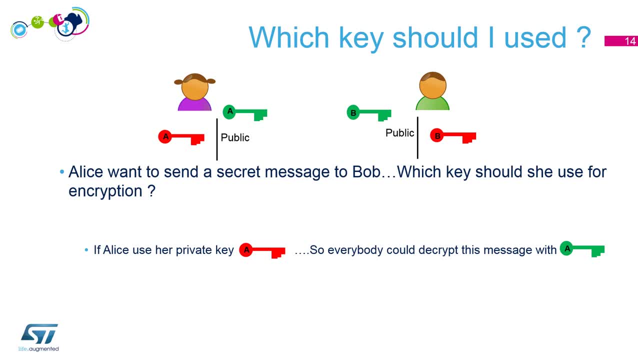 That means the Alice public key. But this key is public, So that means anybody can decrypt it, Even Eve. So where is the confidentiality? Nowhere. That's not the solution. Other possibility: Alice could encrypt with her public key. That means it could be decrypted only with the Alice private key. 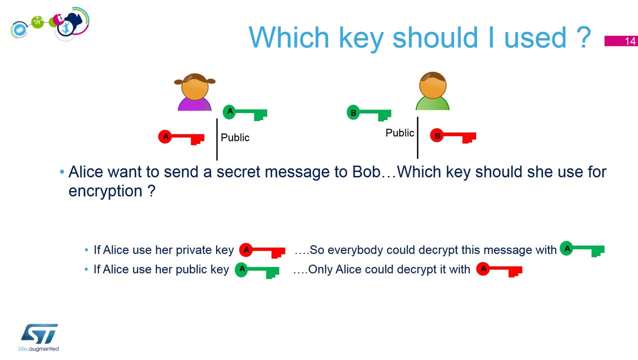 That's not the purpose here. We want Bob to be able to decrypt. So now we've got it. The solution is to use the Bob public key. When Alice encrypts with the Bob public key, only Bob can decrypt the message with the associated private key. 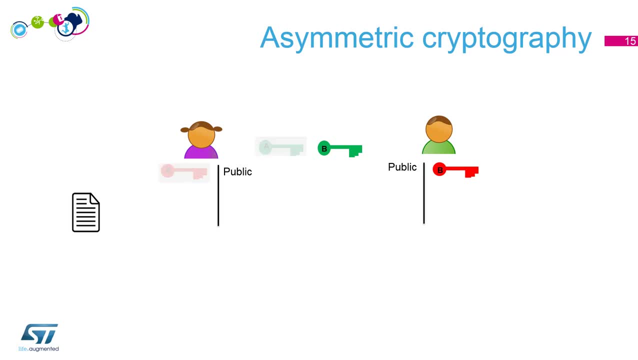 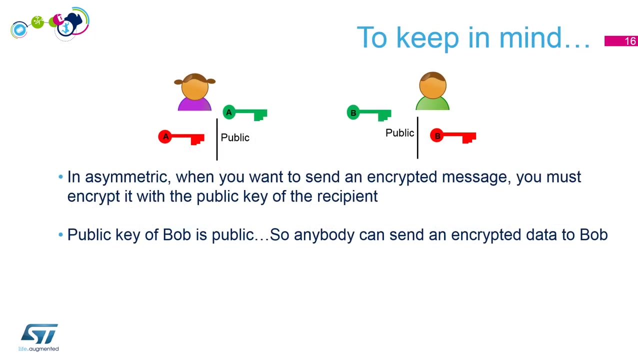 Alice prepares a message, We'll encrypt it with the Bob public key. Then the message is encrypted And only Bob got the associated private key to decrypt this message. So to keep in mind in an asymmetric system when you want to encrypt a message: 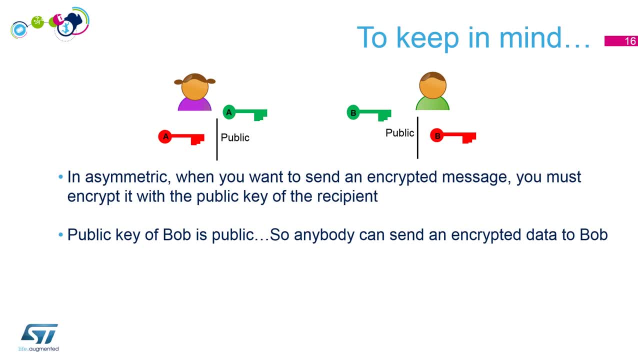 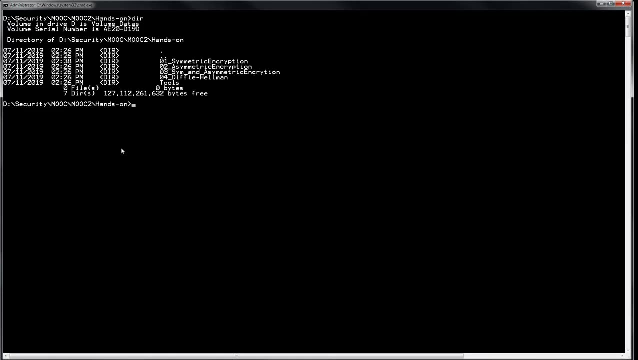 you must do it with the public key of the recipient And also keep in mind public key is public. Anybody can use it or can have access to it. So now let's do a short rundown about this topic. So now we'll do the asymmetric encryption. 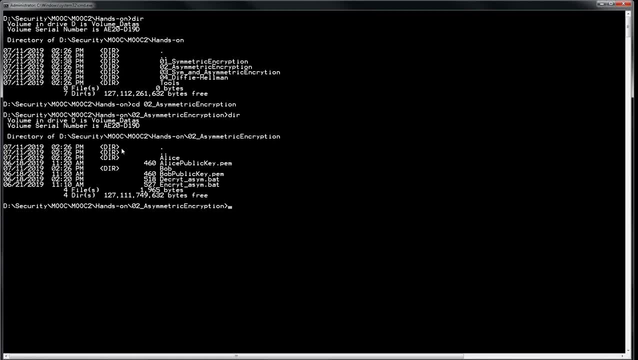 Here we've got a folder Alice and a folder Bob, And this is the private part. I will save for them In the public domain. we've got the Alice public key, the Bob public key and the batch to encrypt or decrypt. Alice got the public key. 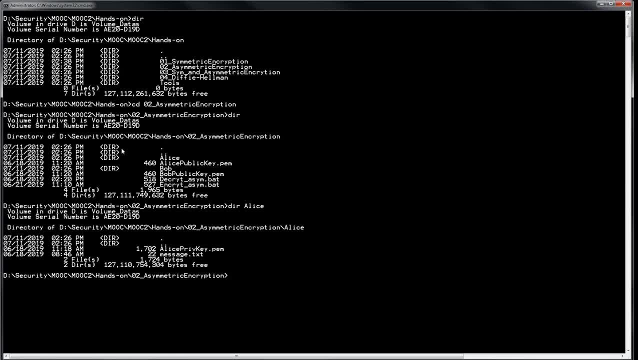 The message she wants to send And she's got the private key associated with the public key that is in the main folder. Bob has his private key, So now let's start the encryption. So we want to encrypt. The first argument will be the key to use. 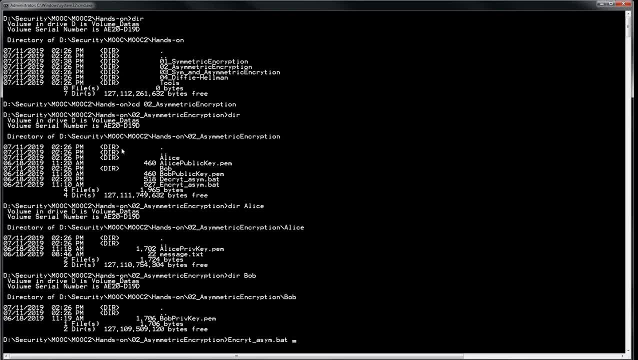 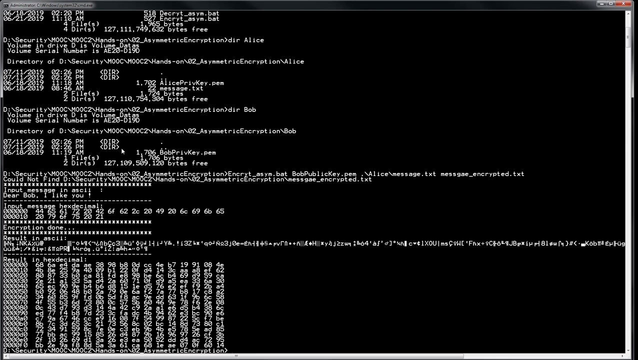 And remember, it's Alice who wants to send something to Bob, So she will encrypt with the Bob public key. Alice wants to encrypt the message. The output file name will be the message encrypted. So let's do this. As you can see, 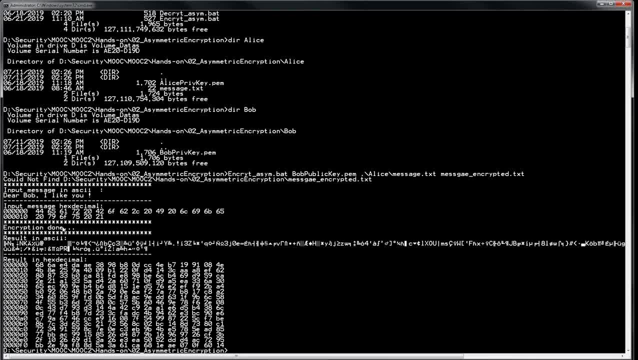 the input message is always the same. Dear Bob, I like you. Encryption is done, You've got huge output data. Now we want to decrypt. It's Bob that will decrypt And he will use his private key to decrypt. So in the Bob folder. 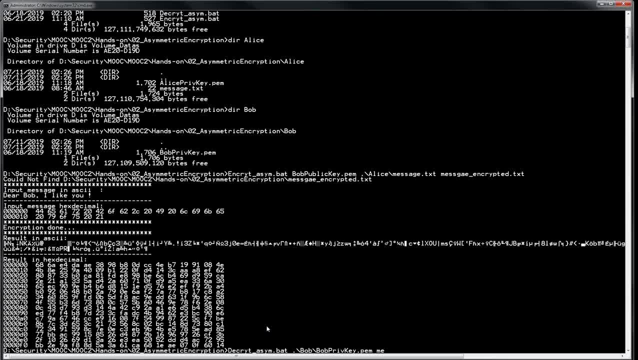 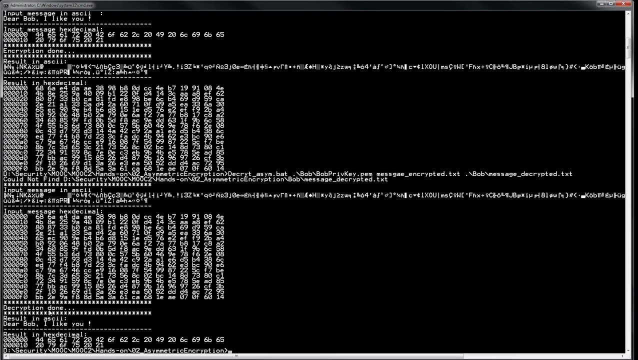 I will use a Bob private key. The input will be the message encrypted And Bob will store the message decrypted. You've got the result here. Bob managed to read the information So he was able to decrypt this. This basic comes on again. 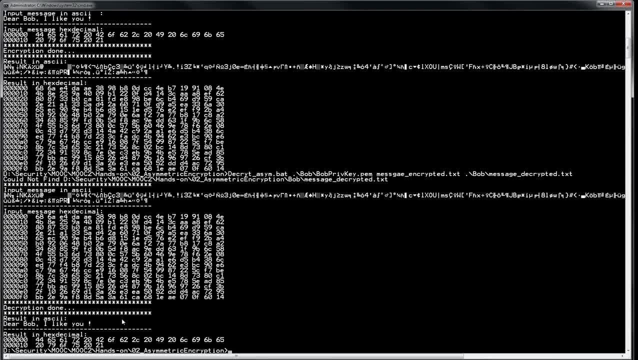 It's just to help you fix ID. If you try to decrypt with other keys and things like that, it won't work. You will often have error of MyScript due to the OpenSSL behind. But here it's just to show you and to fix ID. 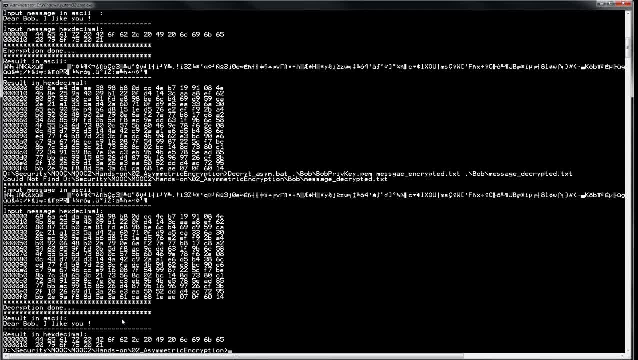 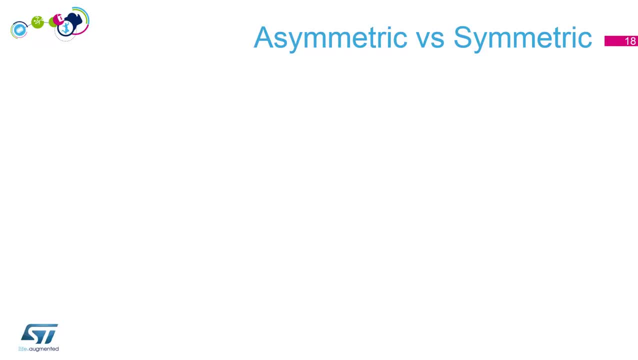 When I want to encrypt something to somebody or for somebody, I would say we should encrypt this data with the public key of the recipient. I hope it's fixed ID. Now we've seen the theory about symmetric encryption and asymmetric encryption- decryption. Let's just remind the advantages. 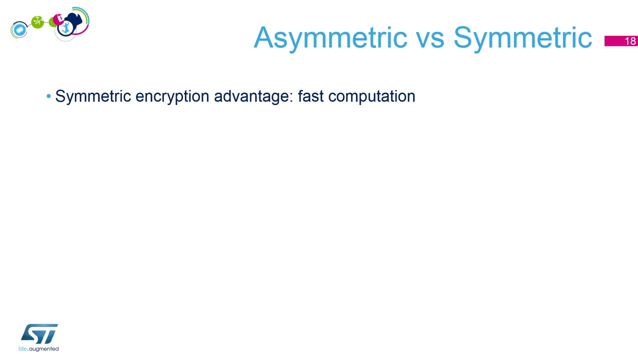 on the drawback for each of them. For the symmetric encryption: the main advantage- fast computation, But the main drawback: you need a shared secret. So before exchanging any data you need to have a shared secret on the both side. For the asymmetric encryption: 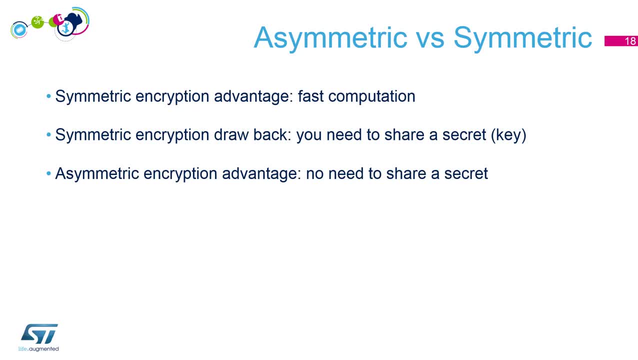 the advantage is that you don't need shared secret, Because you will use a public key to encrypt and you will decrypt with a private key. But it was the slow computation that is your drawback. You can't encrypt or decrypt large data in an efficient way. 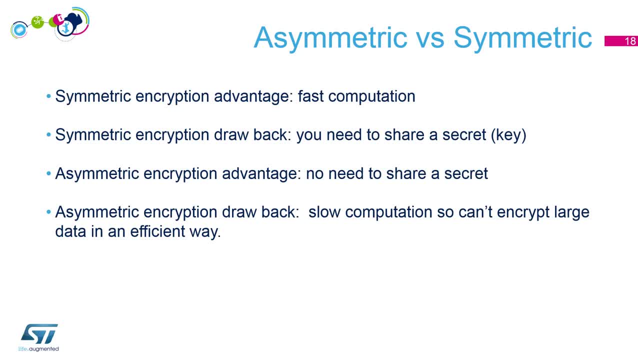 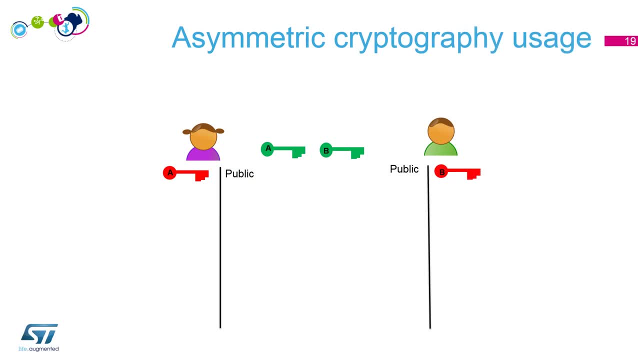 Just reading this, you should think about something: Why we don't combine those both? So let's see how we can do this, And I will say it's a way that we will use asymmetric and symmetric cryptography. What we will do, we will encrypt the shared secret. 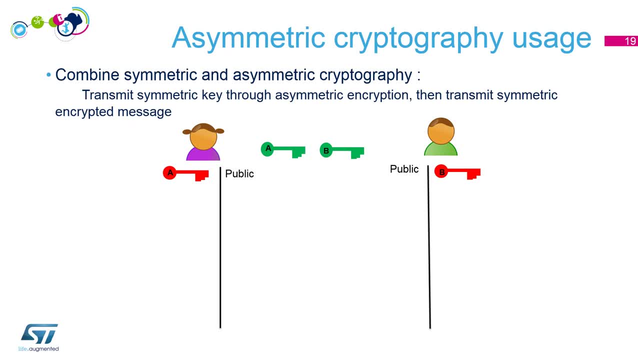 in an asymmetric way, And then we will use this shared secret to encrypt the message. So what will do Alice? Alice write a huge novel for Bob. this time It's a long, long text, And she will decide to encrypt it with a symmetric key. 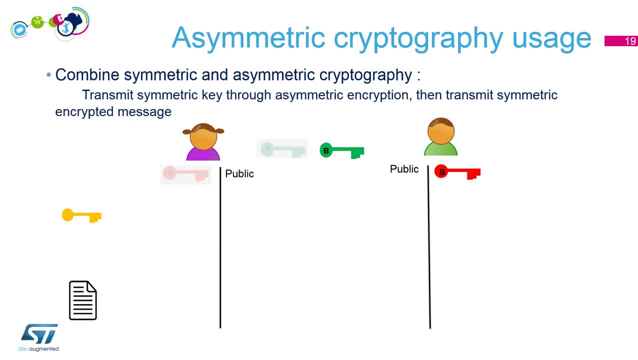 But she want to share this key with Bob And for that she will use asymmetric encryption. So she will encrypt the symmetric key, the golden one, with the public key of Bob And, remember, the only way to decrypt this would be to use the associated private key. 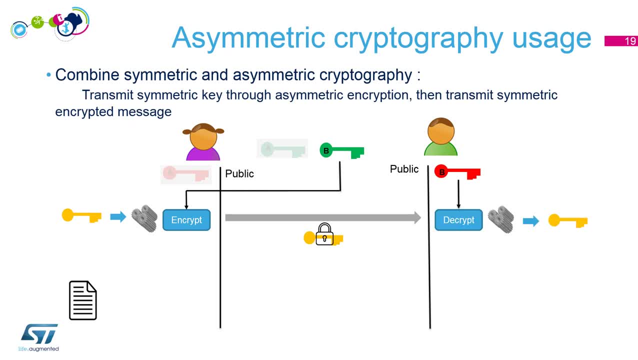 So only Bob can decrypt this content And he can get this golden key. So now we are exactly in the starting of the symmetric encryption. We've got the shared secret, the golden key And we've got data to exchange. So now 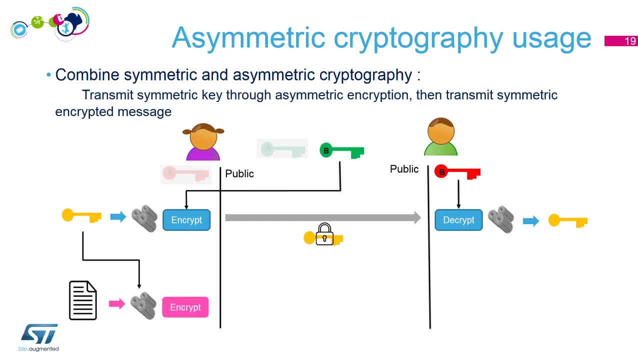 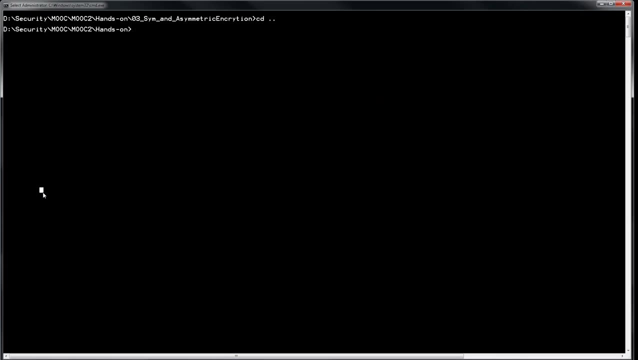 Alice, we just encrypt this document with this golden key, Share it with Bob And Bob can decrypt it, And that's it. Let's see just a short hands-on about this. Ok, now let's continue with a hands-on with combination of symmetric and asymmetric encryption. 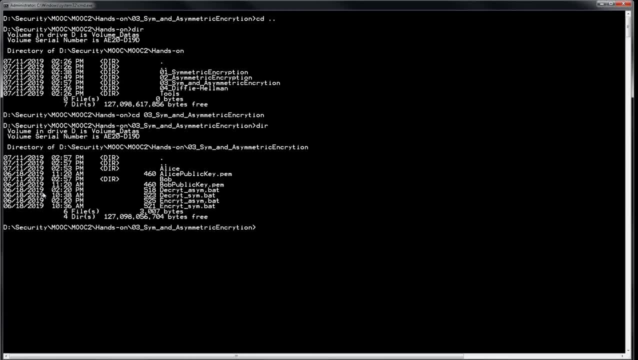 So here you've got some byte files to encrypt, decrypt symmetric or asymmetric way. You've got the public key of Alice and Bob. Alice got a message to send. It's a private key also And a symmetric key value she wants to use. 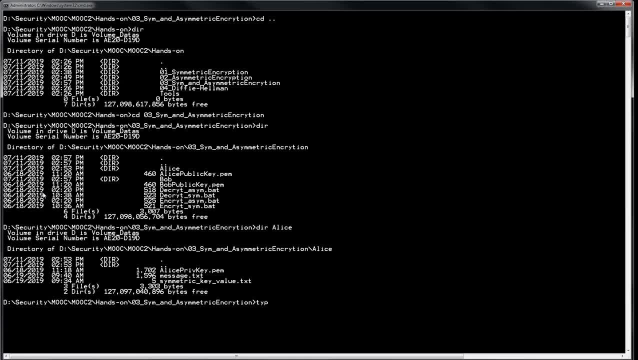 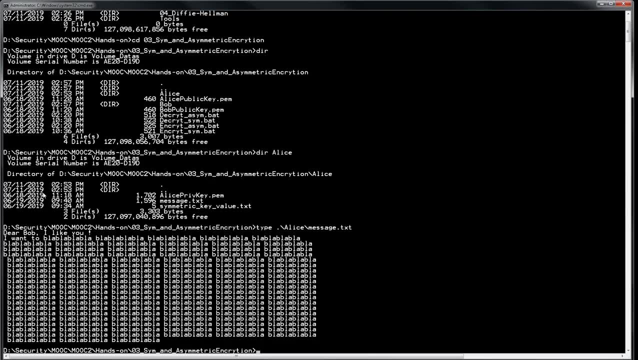 to encrypt this message. So let's check the message of Alice. This time it's a little bit long, So I want to use the symmetric key. I want to use the symmetric encryption to encrypt this data, Not the asymmetric one, because it won't be efficient enough. 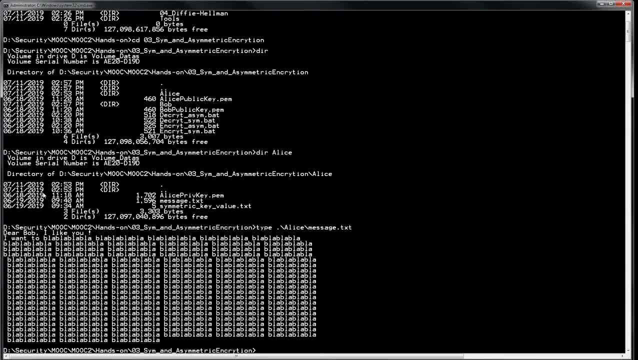 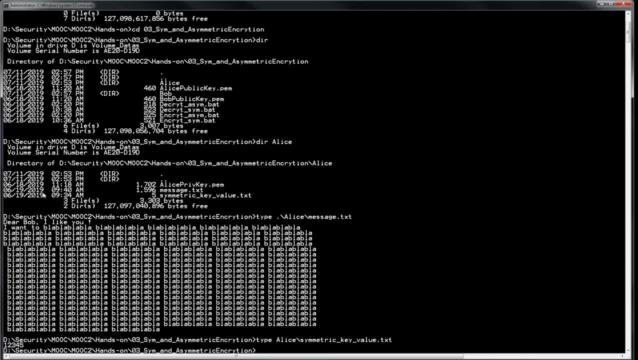 That's not a real case, but let's imagine The symmetric key value that we'd like to use. Alice is 1,, 2,, 3,, 4,, 5.. So the idea is to find a way to send this securely to Bob. 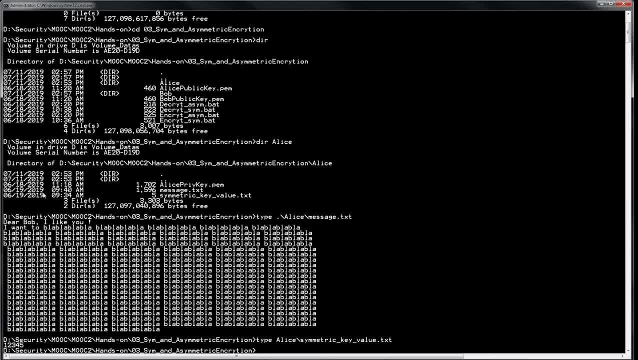 So let's encrypt it with the asymmetric mechanism. So we will encrypt in an asymmetric way. We will encrypt with Bob's public key. That means only Bob with his private key can manage to decrypt this. We will encrypt the Alice symmetric key value. 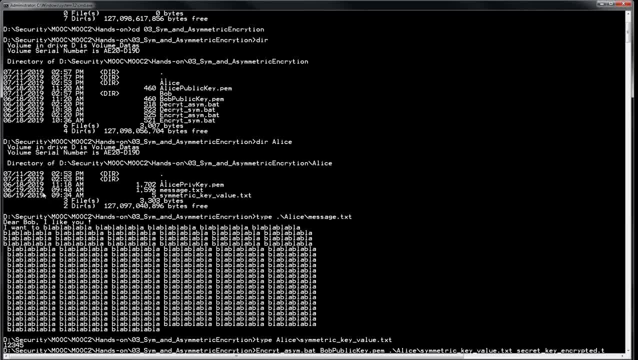 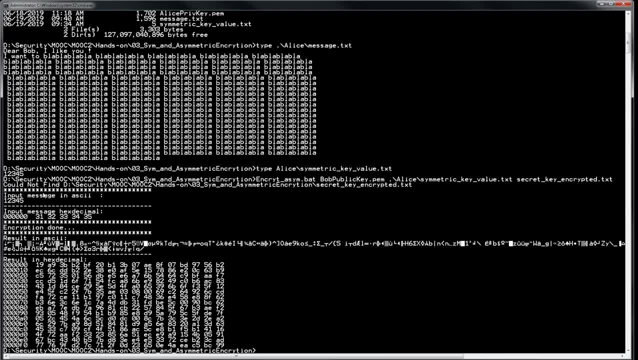 And store it in the file secretkeyencryptedtxt. So that's it We've got. the input message is 1,, 2,, 3,, 4, 5.. So the value we want to use to encrypt And the result is something that you can't. 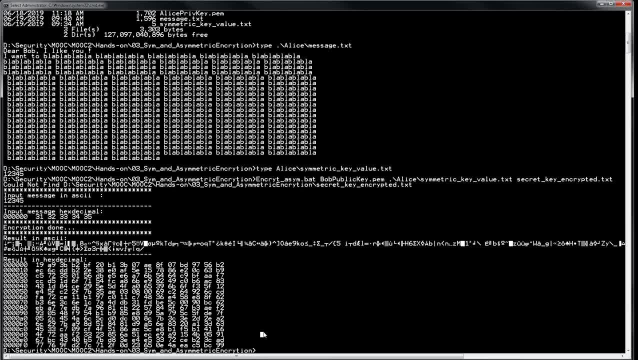 I would say: understand or you can't use. Now Bob will decrypt this secret value encrypted recently, So we will decrypt, still in an asymmetric way. For that Bob will use his private key. We will use the secretkeyencryptedtxt And Bob will store it. 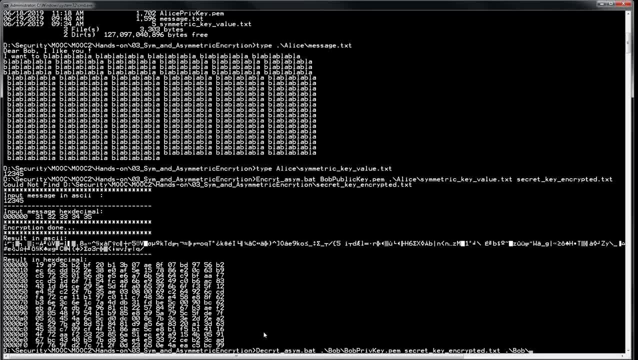 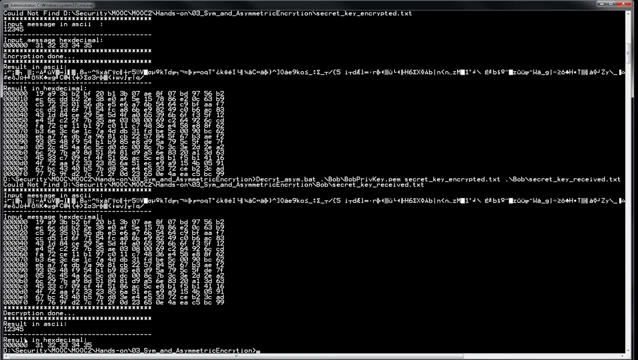 in his personal folder. So, as you can see, he managed to get the value 1,, 2,, 3,, 4, 5.. So, in a secure way, we managed to share something, We managed to share the value of the key. 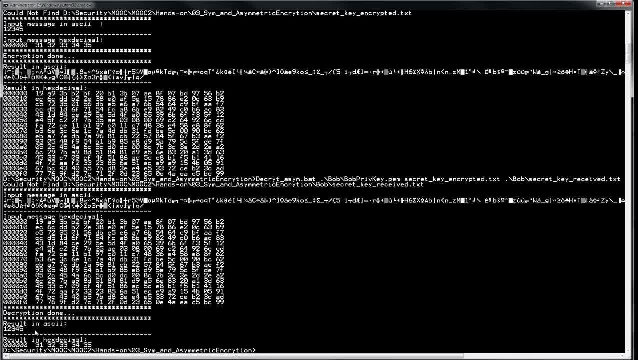 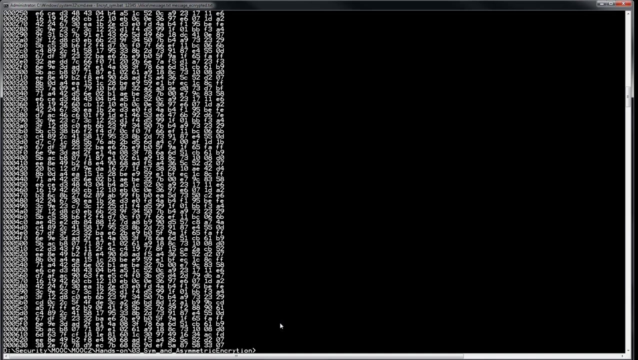 that Alice now will use to encrypt the file in a secure way. So this time we will encrypt, but in an asymmetric way. We are using the key value where we agreed. So she takes the message, The message, encrypted. That's it, Okay. 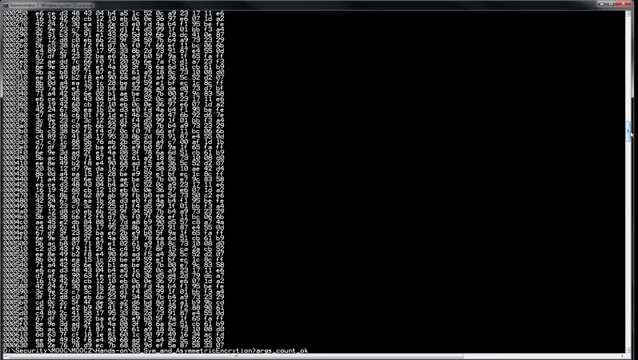 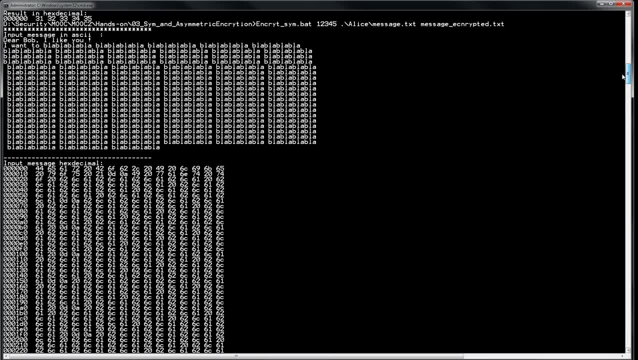 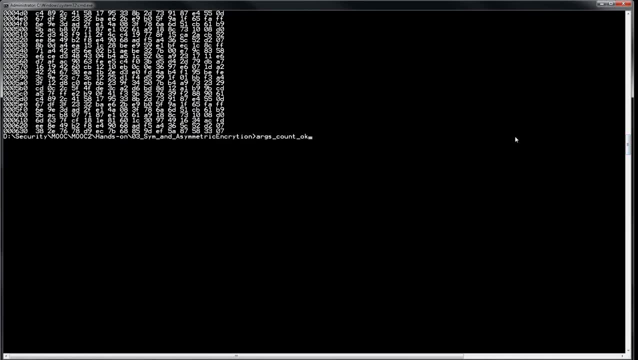 So here you can see, there is many, many information This is due to. I just show you the result in husky and also in hexadecimal. So, as you can see, Okay, It was well encrypted, I would say. So now it's Bob that will try to decrypt this. 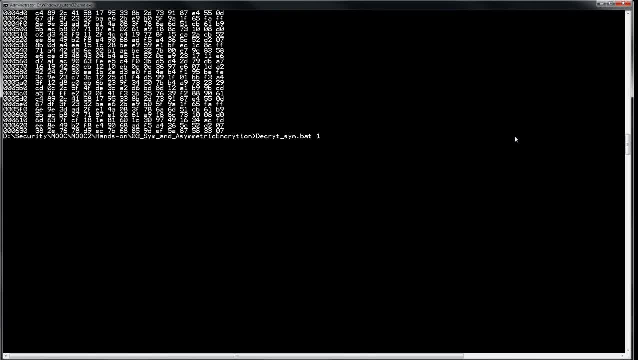 So he will decrypt in an asymmetric way. He knows that the key value to use is 1,, 2,, 3,, 4, 5.. Because he received this value previously, He will use the message encrypted And he will store it. 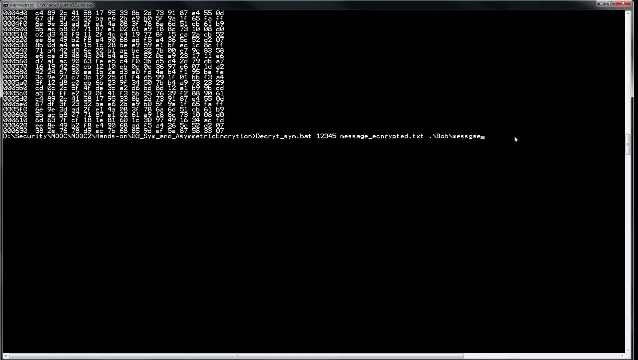 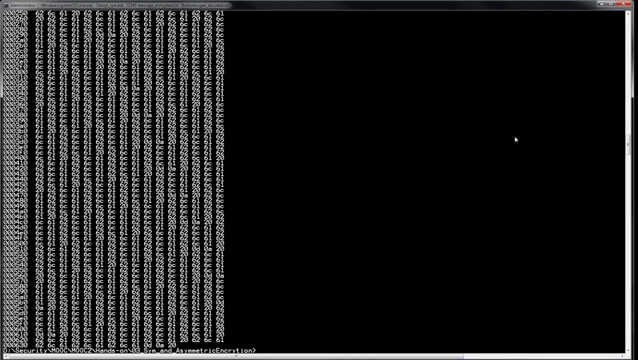 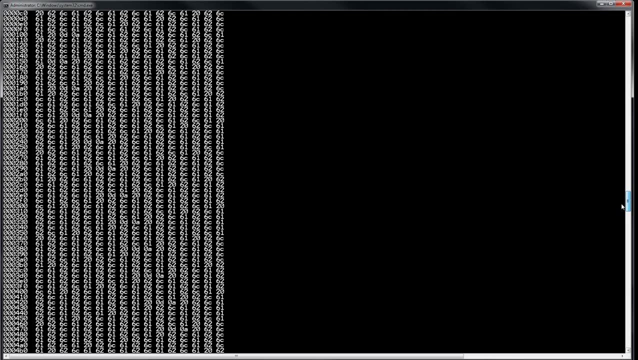 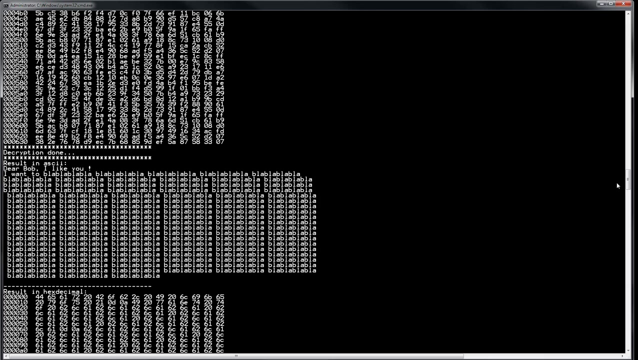 in his folder. Sorry for the sound. So here we can see that Bob recover the value. So here you've got the main schematics. You are using asymmetric encryption to have a shared data between the both sides, And now you can use this. 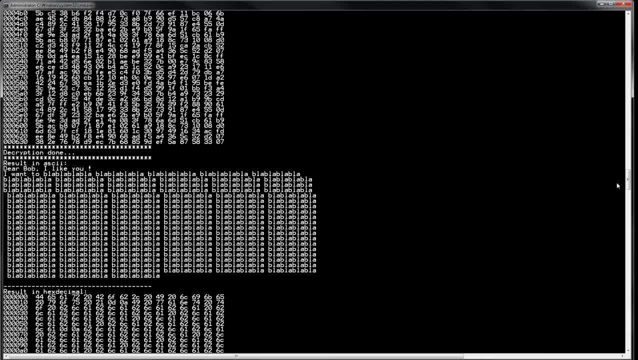 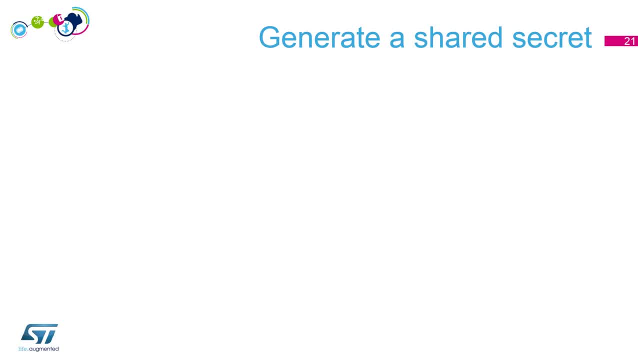 shared secret to encrypt in a symmetric way. I hope it helps you fix highly. Now I would like to introduce you another way to create a shared data in a secure way. So this is possible thanks to an algorithm called Diffie-Hellman. 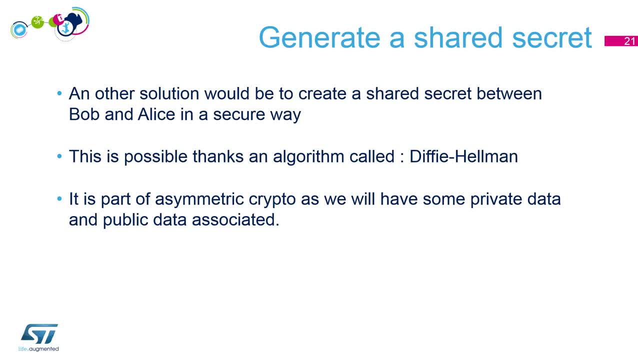 It's part of asymmetric cryptography because it uses some public data and private data associated, But it's different from the previous scheme we've seen together. To explain this theory, I will use some color mixing example a little bit different from the previous one I will deal with. 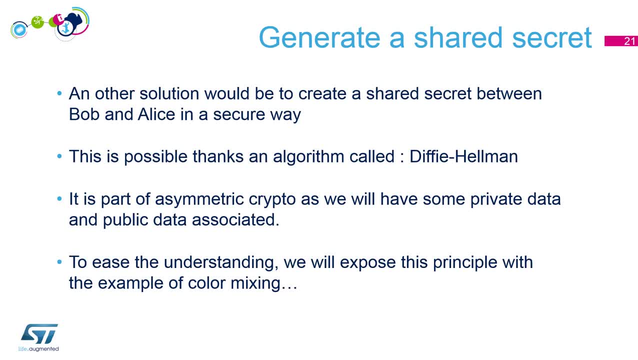 the details about mathematicals in the next part. So for the moment it's really a little bit different from the previous, but I think it will help you understanding this algorithm. So first, Bob and Alice will agree on one color. This color is here yellow. 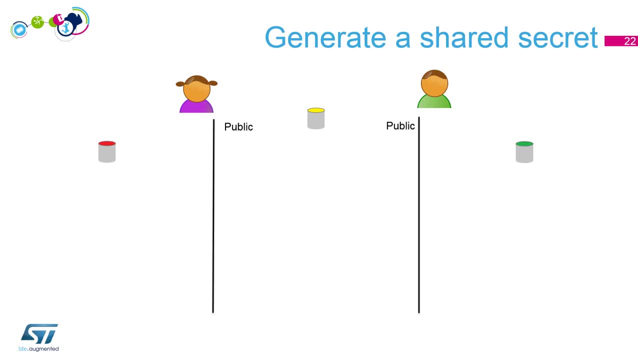 Then they will choose a private color. So Alice choose the red and Bob the green, And Alice will take the public color, so this yellow, and will mix it with this private color. She will have some orange now and she will send this to Bob. 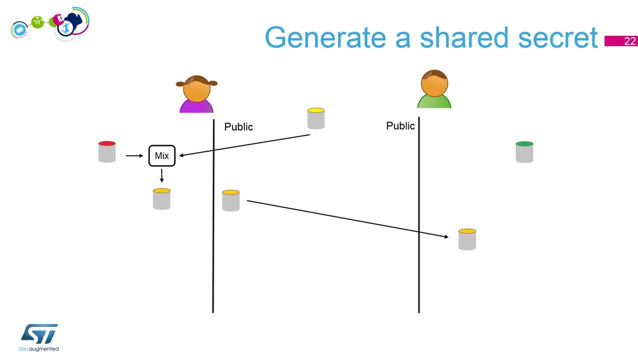 One thing important is, even if you've got the orange and the yellow, you can't find out the red color. It's impossible to extract it because they are mixed together in this painting and you can't just extract it. It's not possible, Just think. 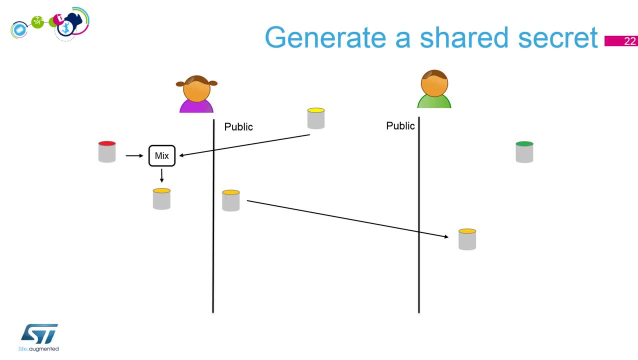 that even if you've got the yellow and the orange, you can't find the red. So Bob will do the symmetric things. He take the yellow, mix it with the green and will have some blue color and will send it to Alice. And again, even if you've got 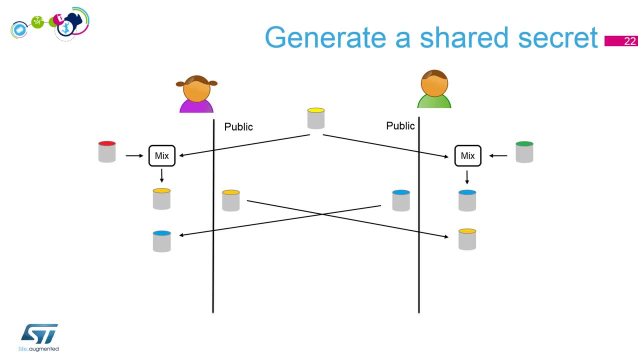 the yellow and the blue. you can't extract the green from this. It's not possible. So now Alice will take this blue and will mix it with this private color again. And what does she have? The same with the orange. I mean, take the orange. 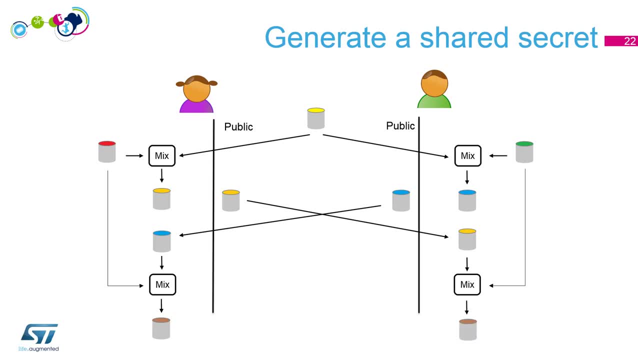 and mix it with this private color, it will have exactly the same brown. So from the public part we have seen the yellow, the orange, which is a kind of a way to hide the red of Alice, and we've got the blue, which is a kind to hide. 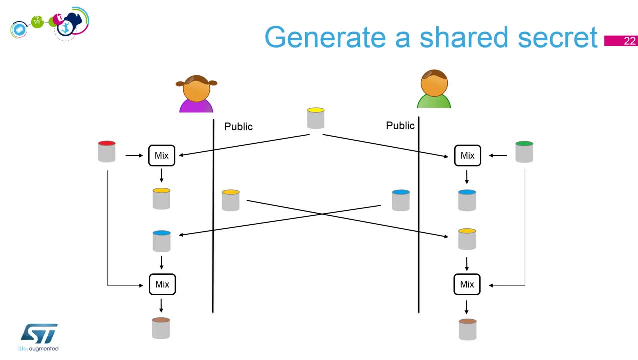 the green of Bob, and they share this on each side. now they have exactly the same brown color and it's the same with the pink, which is the same with the yellow, which is the brown, and the blue is the same with the blue, which is the orange. 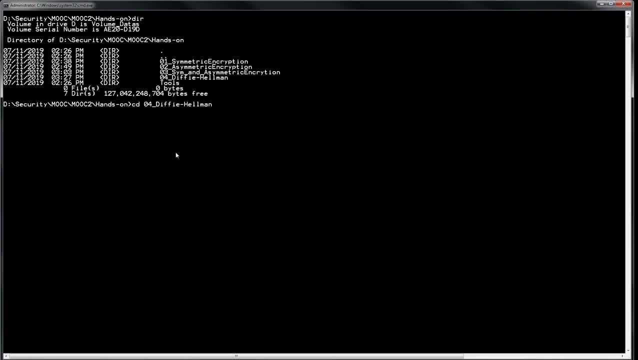 which is the pink and it's the blue. you get three script, sorry. so we've got one to generate the common color, one who allow you to choose a private color and mix it with the common color, and another one to generate the secret. so first we should select a common color. let's call: 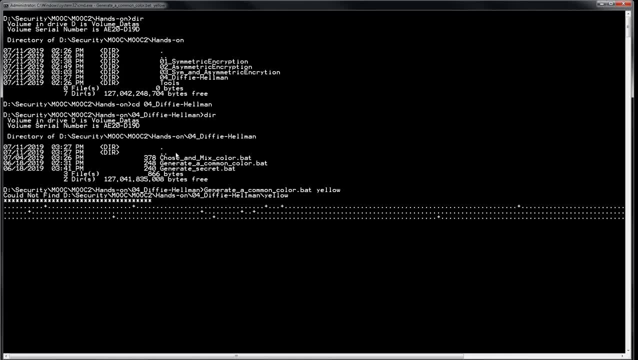 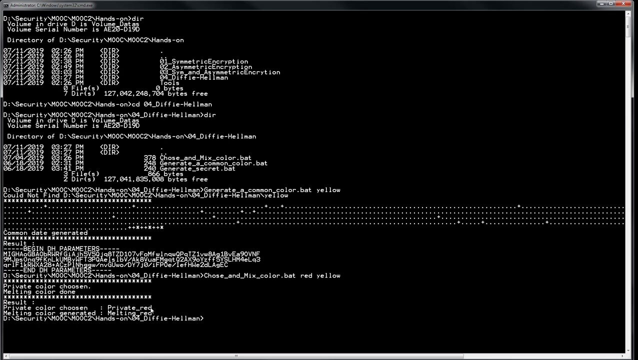 it yellow, so take a while, but it's okay. now we managed to generate, I will say, our yellow color. now Alice will choose its private color and we mix it with this yellow, so she choose a mixed color. she will choose some red and want to mix it with yellow. so what is generated- the private color chosen- is private red and 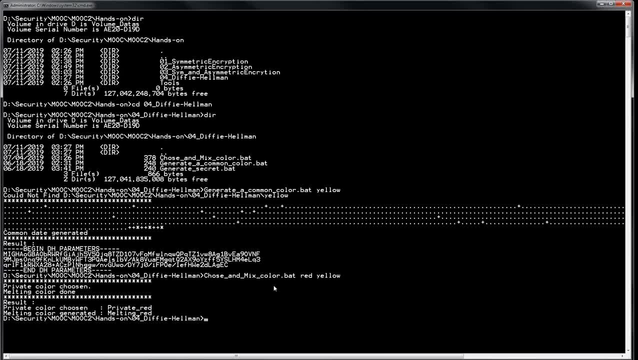 the melting colors, which is the result of the private colors, and the yellow is a melting red. if you've got the melting red and the yellow, you can't find any information about the private red. now, Bob will do the same or I will do it: the symmetric. 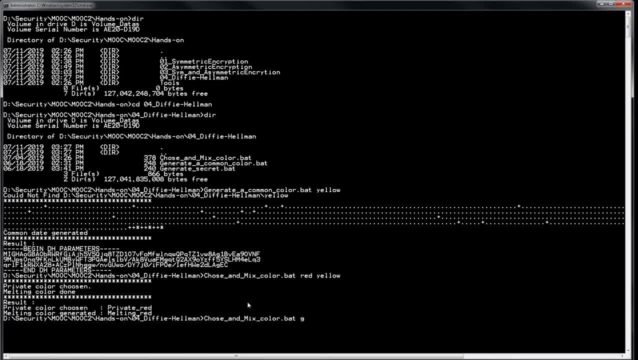 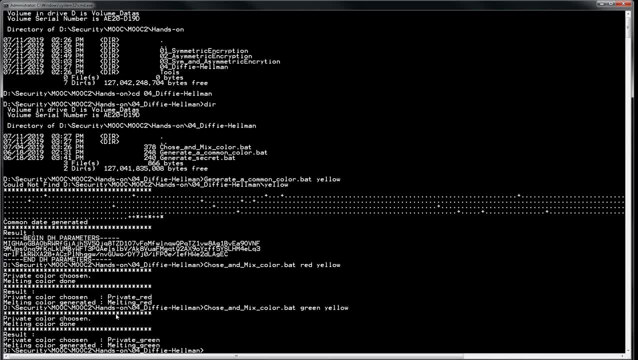 way. so we choose and mix colors. we will choose green and mix it with yellow, so we've got the private green of Bob on the melting grid, which is a result of the private green melting with the yellow. now we can generate the secret Alice started, so she generates a secret to do. that she will use is her private. 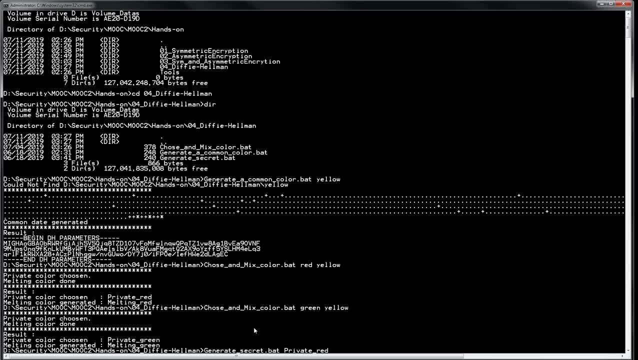 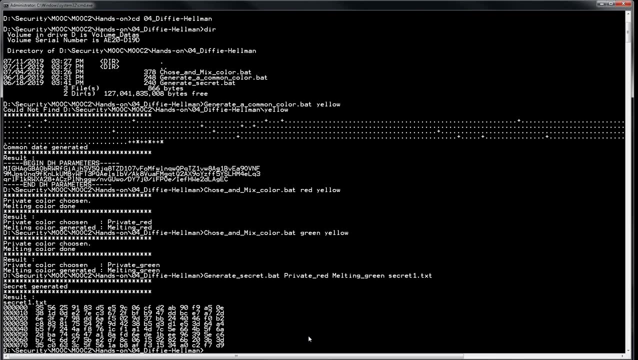 color, so the private red, and she will mix it with the melting green she received from Bob. this is a secret one, so we've got a value, we've got a secret generated under this value symmetrically. Bob will do the same. he will generate a secret with its private green and will use a melting red. I put it in the 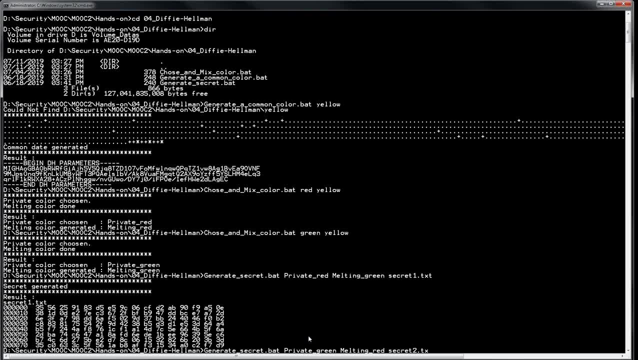 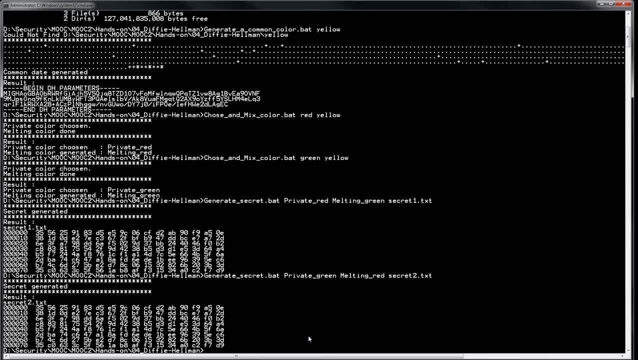 secret to xd file and if you've compared the both are equal. we managed to cut some shared secret from the both side without sharing any secrets, so I hope it's helped you fix, Heidi. I, I know that differently. it's not so obvious to, But here we've got some things that just show you with some command and you can do many tries with it. 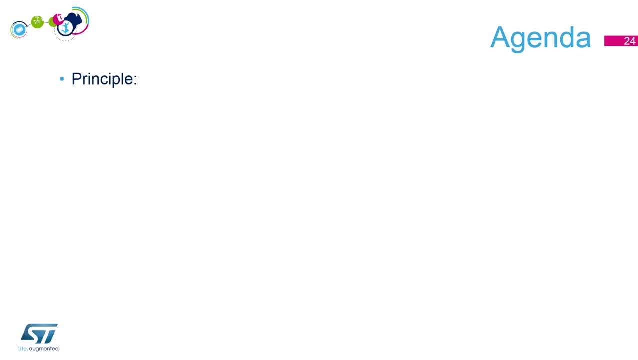 Where do we stand now? Let's check the agenda. The principle we have seen together: symmetric encryption-decryption theory: You remember you use the same key to encrypt and to decrypt. Asymmetric encryption-decryption theory. this time you are using the public key of the recipient to encrypt.